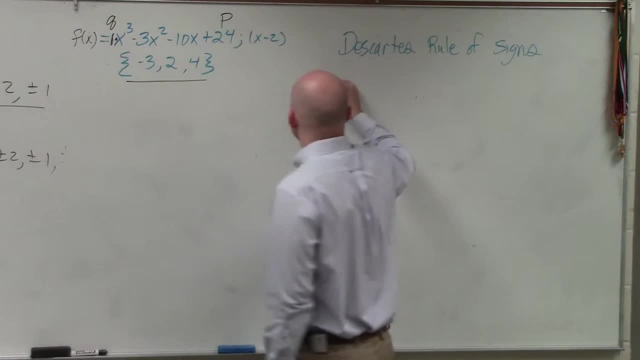 So the first step goes like this: To find the number of real positive, all you simply do is take your function f of x And you determine the number of sign changes between the terms. A sign change means that the term is going from positive to negative or negative to positive. So in this case I have two sign changes. Would everybody agree with me? 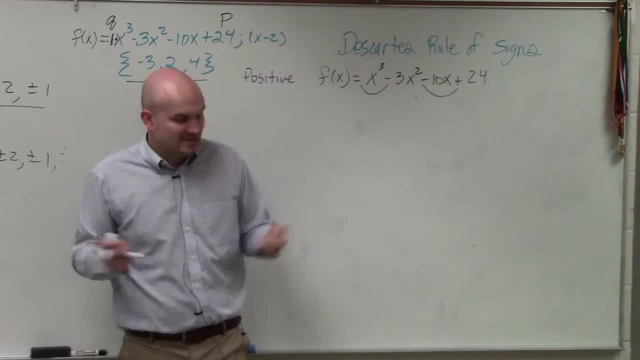 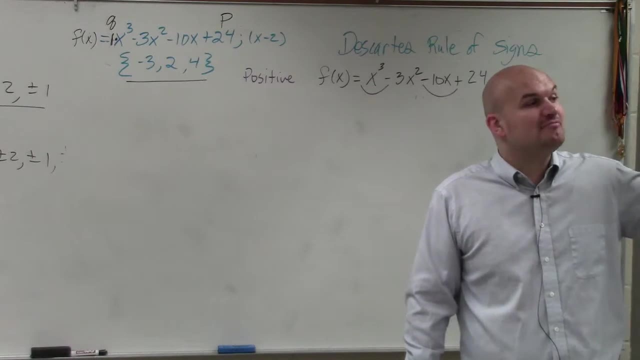 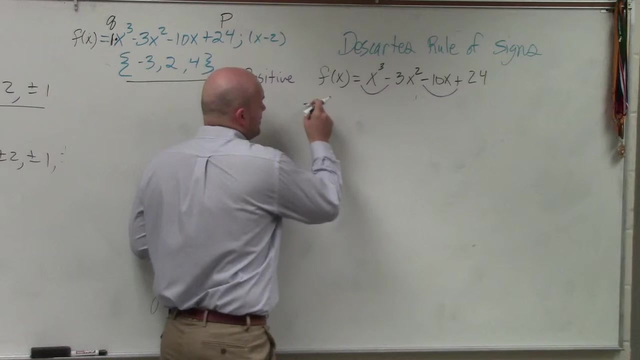 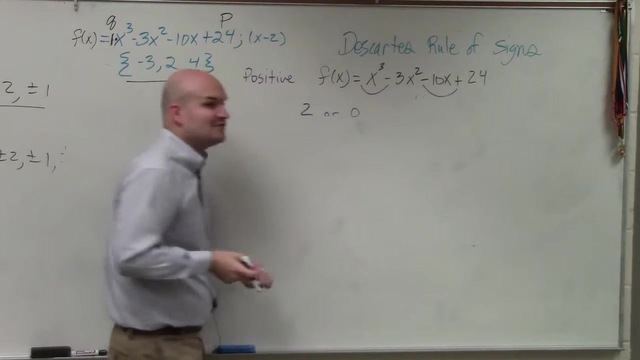 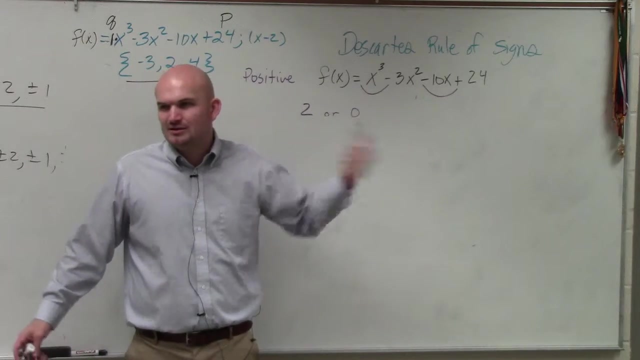 Now Descartes' rule of sines. this is kind of confusing, but this is just his rule. Descartes' rule of sines states that the number of sign changes minus an even number is the number of possible positive Or negative real zeros. So how many sign changes do I have Two? What's an even number? I can subtract from two, Two. So two minus two is Zero. You could subtract four, but four would give you negative two, right? Can you have negative two of something Like an amount of numbers? No, right, You can't have like. so it's not really going to work in this case. 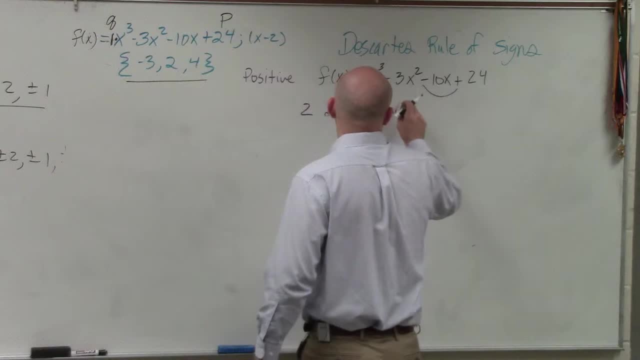 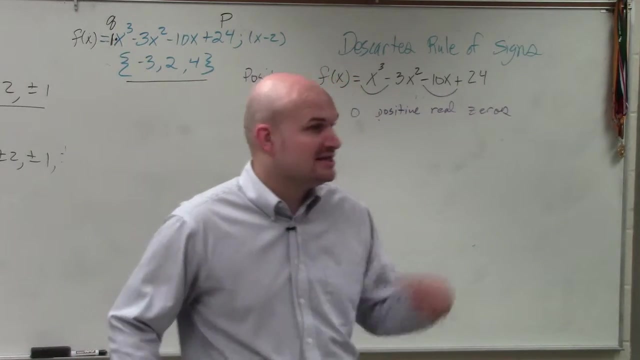 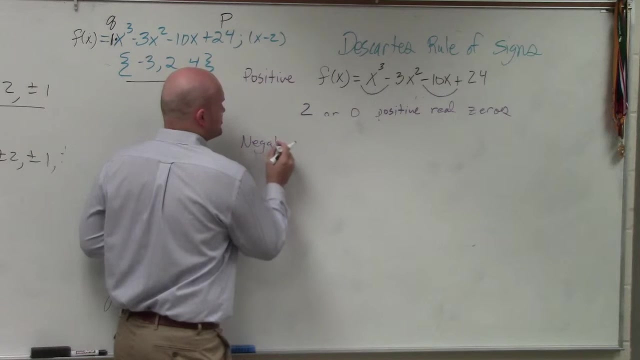 So it's two or zero positive Real zeros. Okay, again, it doesn't tell you how many exactly positive real zeros, It's just telling you it's going to be one or the other. Then the next one is to find the negative. This is the one where students usually have trouble. 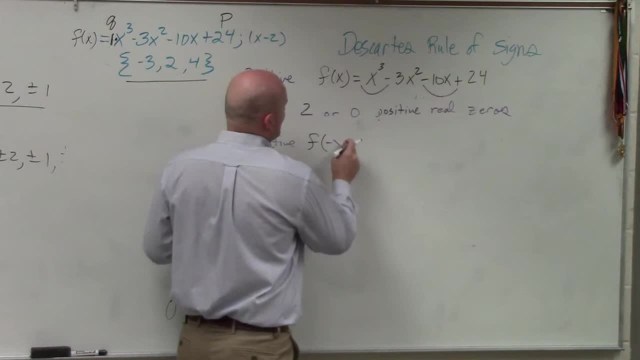 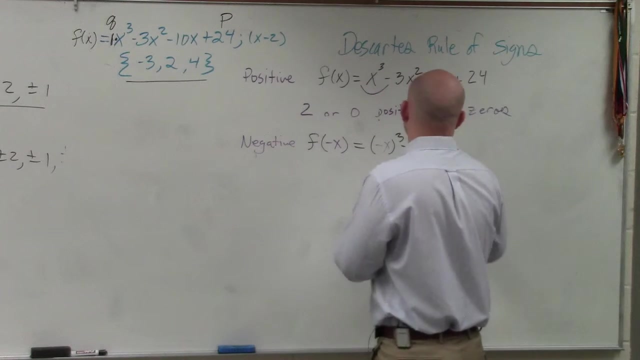 Instead of doing f of x, you're now going to use f of negative x. So now, wherever there's an x, I'm going to replace that with a negative x. Does everybody see what I mathematically did? Yes, 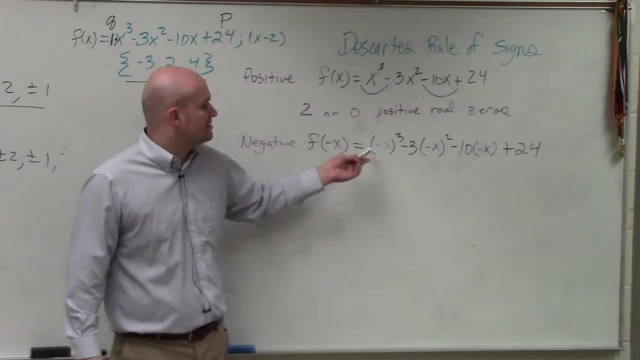 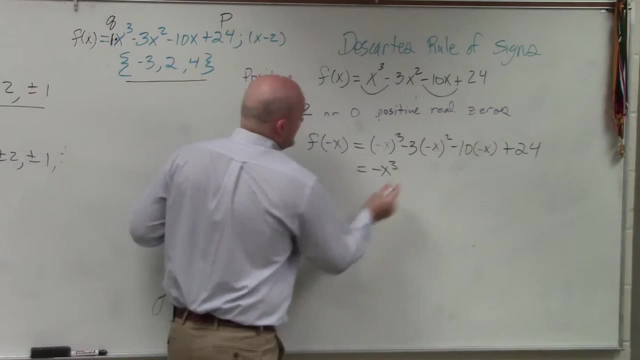 Okay, So now we just need to- now we've got to simplify this. So anytime we have a negative number raised to an odd power, that's always going to still be negative. Anytime you have a negative number raised to an even power, that's going to become positive. 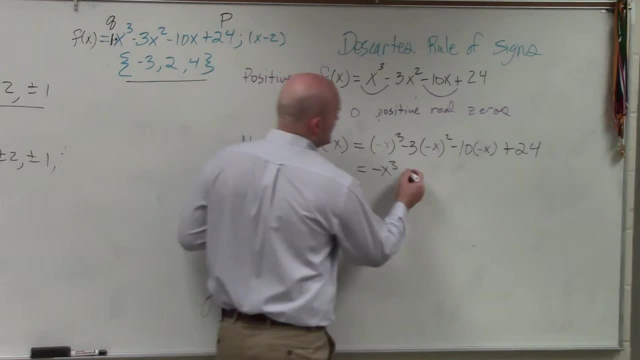 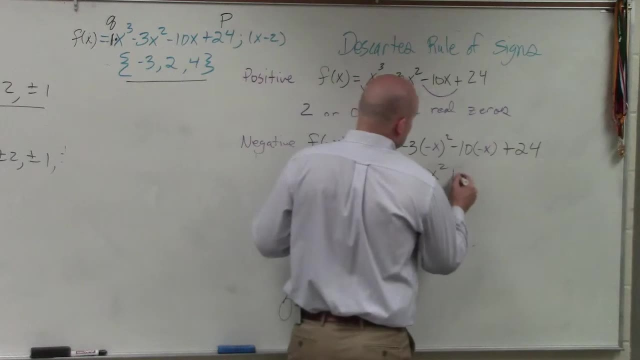 So negative x cubed is now positive x cubed. Positive x cubed times negative three is a negative three x squared And negative 10x times negative x. or negative 10 times negative x is now a positive 10x. 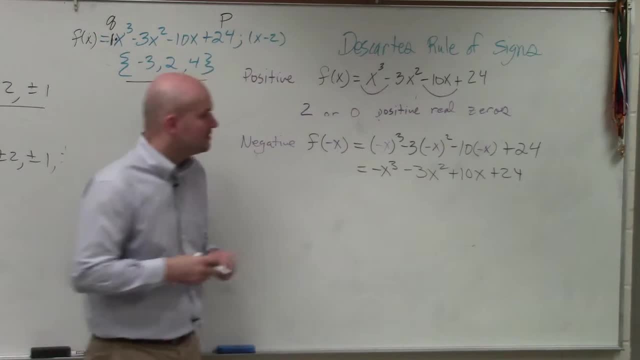 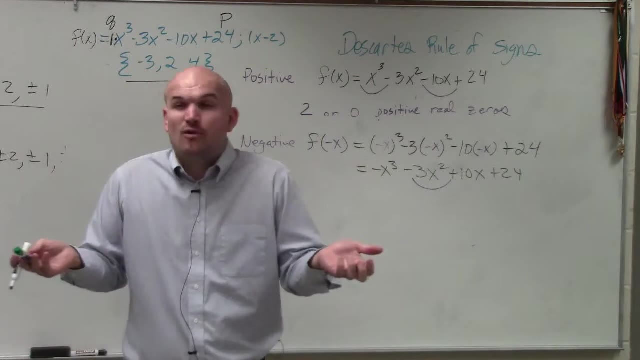 And then plus 24.. Okay, Again, we want to determine the number of sign changes. Number of sign changes is one. Can we subtract a one, Or can we subtract an even number from one and still have a positive number? No, 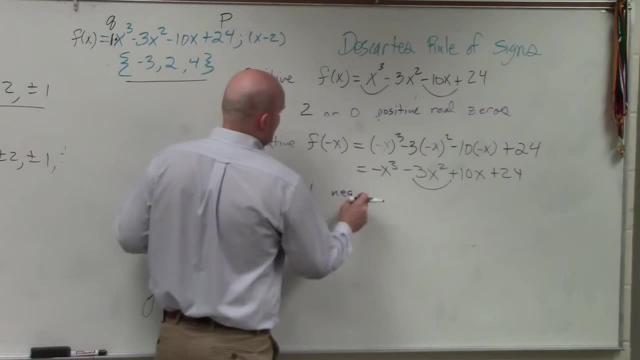 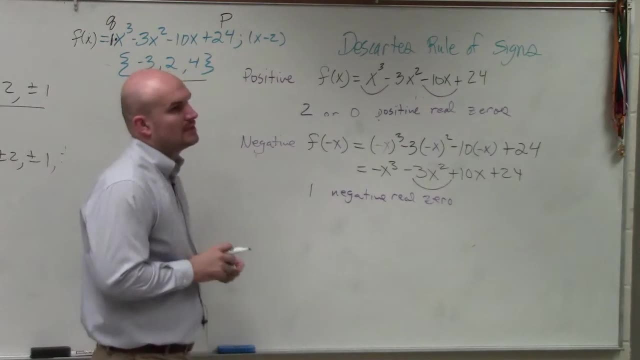 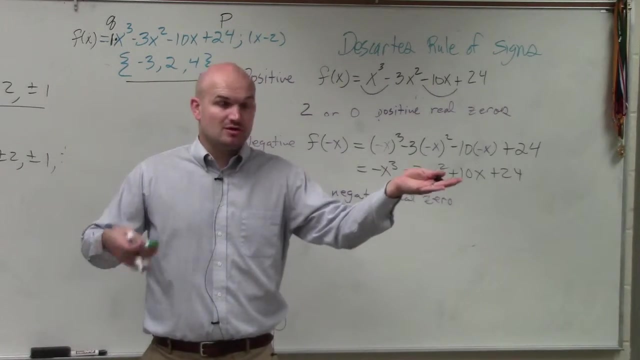 So therefore, for negative, there is one negative real zero. Okay, Now here's where it kind of gets confusing. For quadratics, we either had real solutions or complex solutions, right, Yes, Yes, But remember for 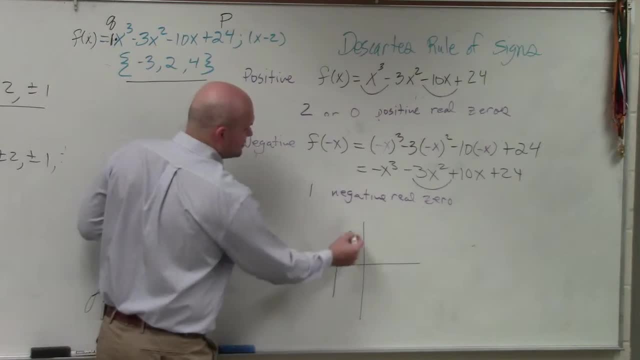 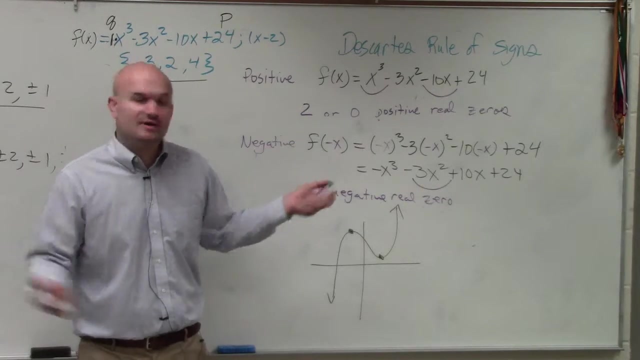 Cubics. it's possible to have a real solution and then have two complex right, Because how many? What's the degree of this polynomial Three right? There's two turning points, so the degree is three. How many, However, how many real solutions are there? 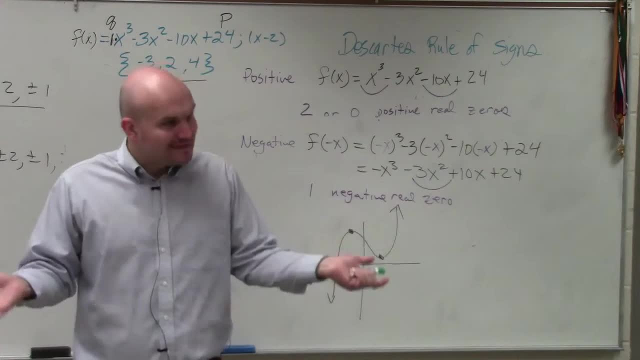 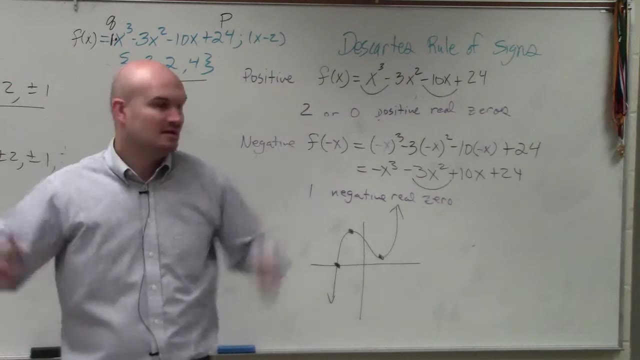 There's only one. So what do the other two solutions have to be Complex, right? So when you have polynomials to a higher power than two, it's possible to have real and complex. So to find the number of complex, I like to use a table. 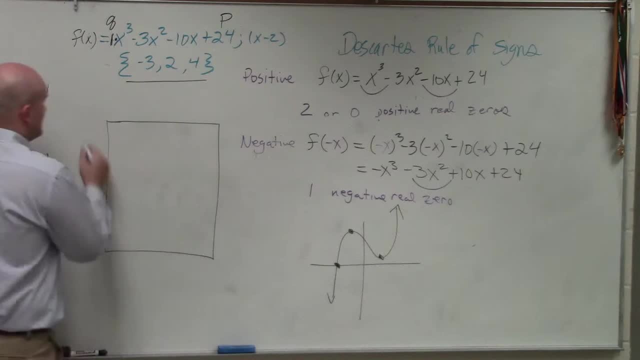 And the table I do is: here Am I getting? How do I say it? Okay, So I can have positive zeros, I can have negative zeros, I can have complex zeros And then I have the total. All right, So 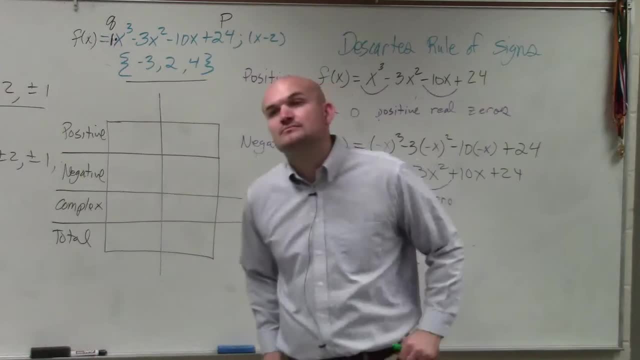 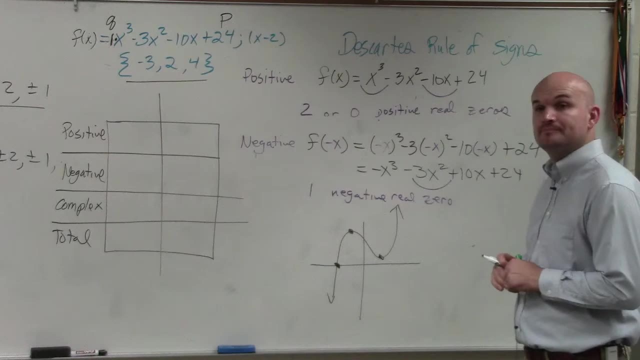 the number of positive zeros? Yes, Santana, I'm sorry. Where This one? Well, this is negative x squared. So that's negative x times negative x, which is positive x squared. Positive x squared times negative three would give you negative three x squared. 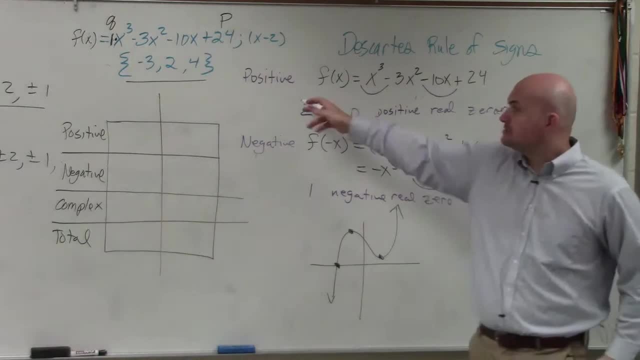 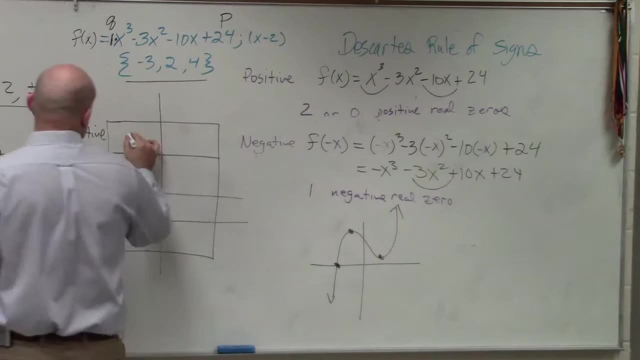 Does that make sense? All right, So the positive: How many possible positive real solutions? do I have Two or zero? So that's why I did two columns. How about the number of negatives? do I have One right?